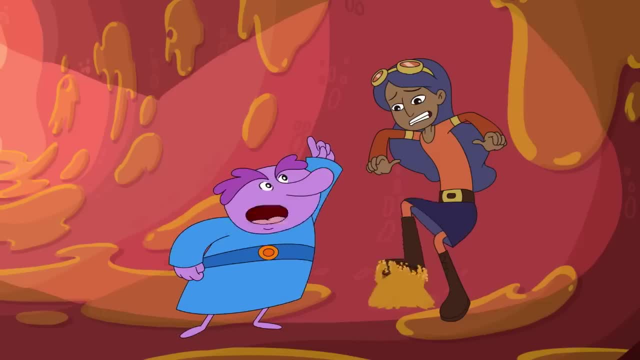 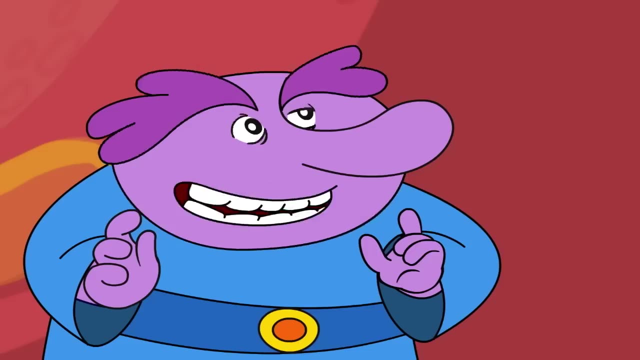 You mean this glorious earwax produced by the ear canal? Nasty earwax is more like it Hardly. Earwax contains chemicals to fight off infections that could hurt the skin here in the ear canal and traps dirt to help keep it clean. 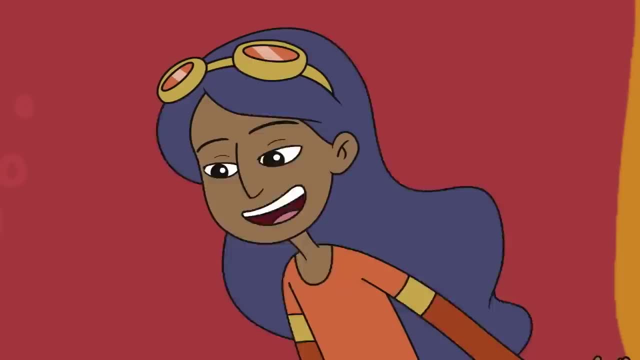 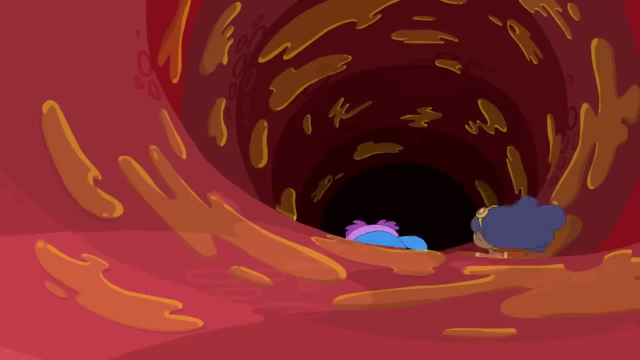 OK, fighting infection and keeping the ear canal clean is important stuff. Oh yeah, Also, earwax will help us slide down the ear canal Woo-hoo-hoo To the middle ear, Where we find the eardrum. 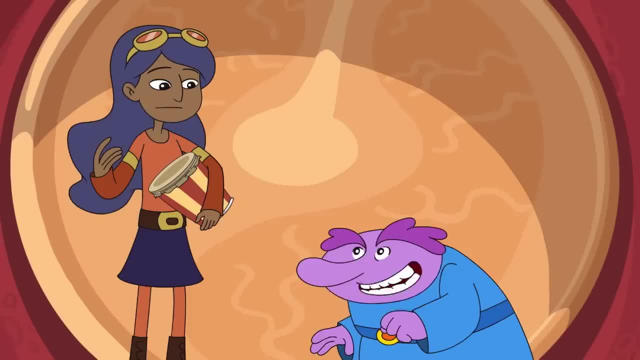 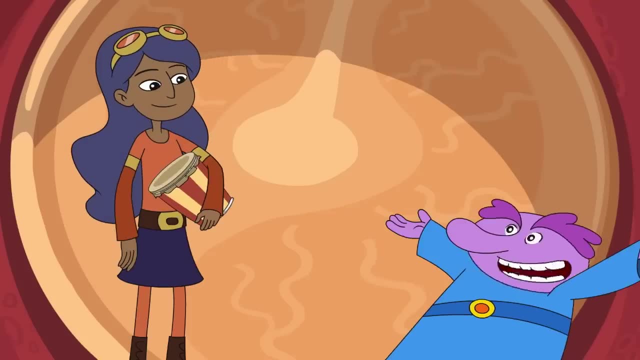 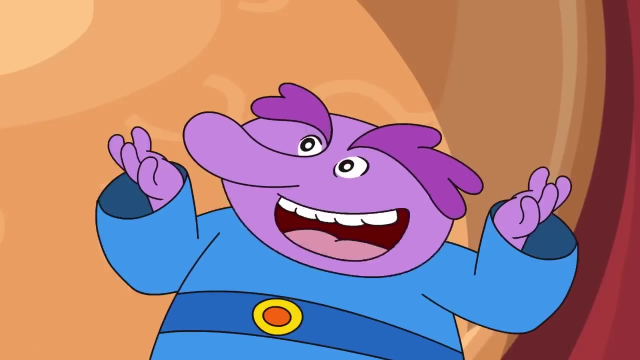 Quietly, my dear Chloe, The eardrum is a very sensitive instrument. Ah, much better. Like my bongo drum, The eardrum is a thin piece of tightly stretched skin. Do they work the same? Very much the same and also different. 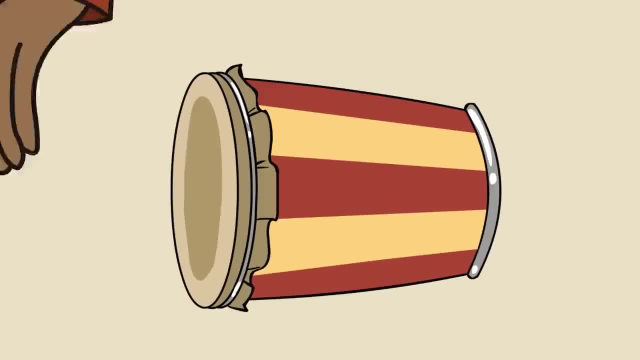 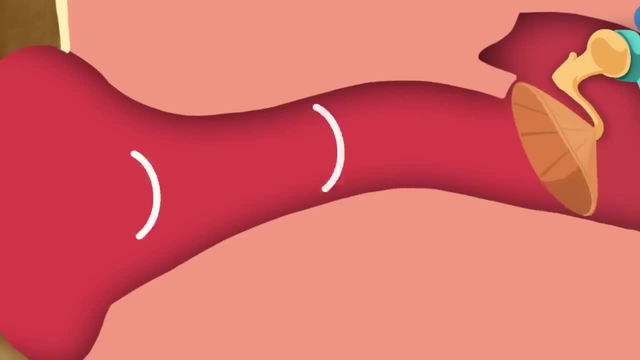 Such a nerve thing to say. Explain: A musical drum makes sound when we hit it, But no one's hitting the drum. in your ear, The sound waves that your outer ear collected cause it to vibrate. Sound waves vibrate the eardrum. 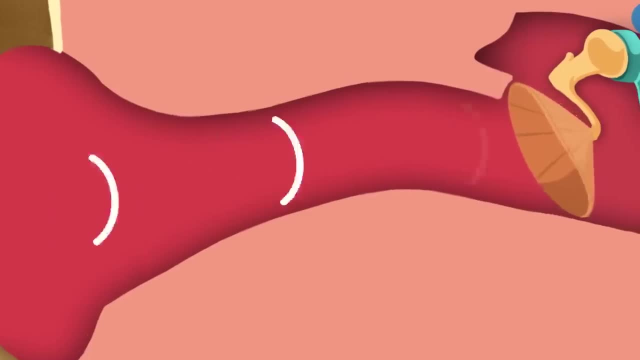 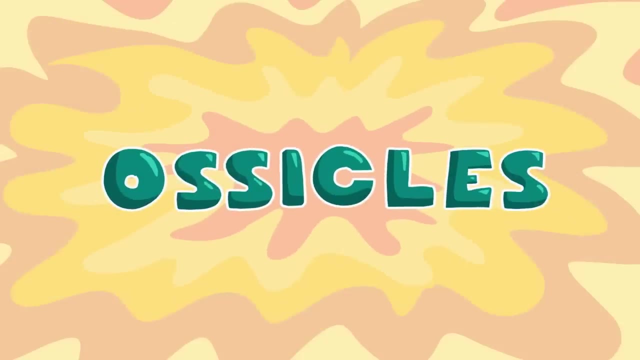 Got it. What happens next? When the eardrum vibrates, it moves a set of three tiny bones on the other side called ossicles, Ossicles. That sounds like a drum beat: Ossicles, ossicles, ossicles. 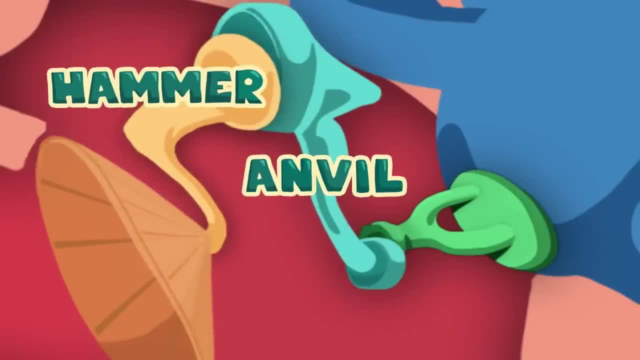 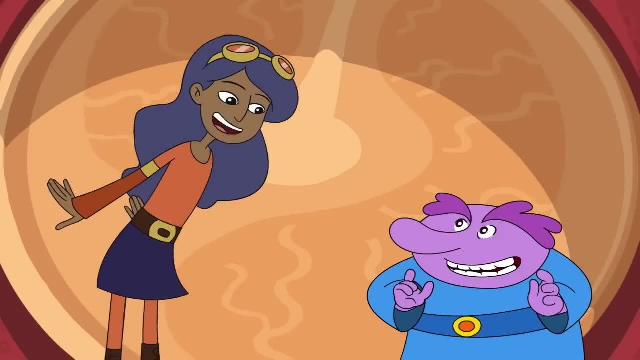 The three ossicle bones are called the hammer, the anvil and the stirrup. Huh, Those bones sort of look like those things, But the sound's journey to the brain isn't over yet, is it Not even close? 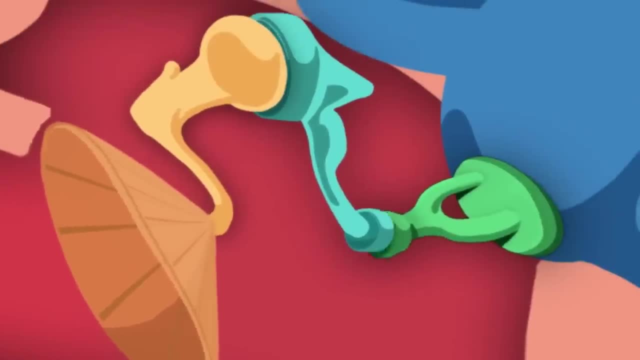 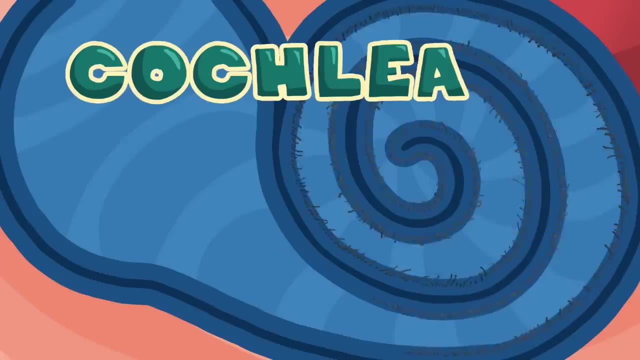 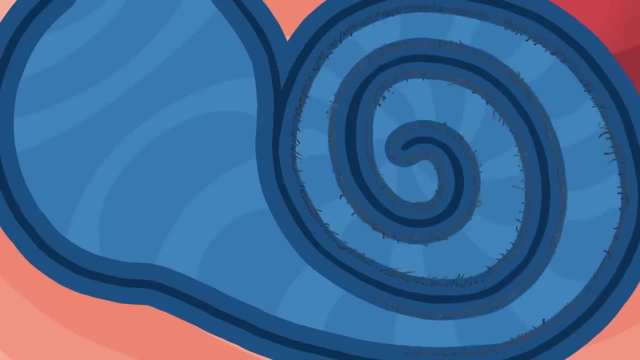 The cochlea is a small curled tube filled with liquid. The vibration of the ossicles create waves in the liquid. in the cochlea Are those little hairs. I see, I'm so happy you asked. The cochlea is lined with tiny hairs.